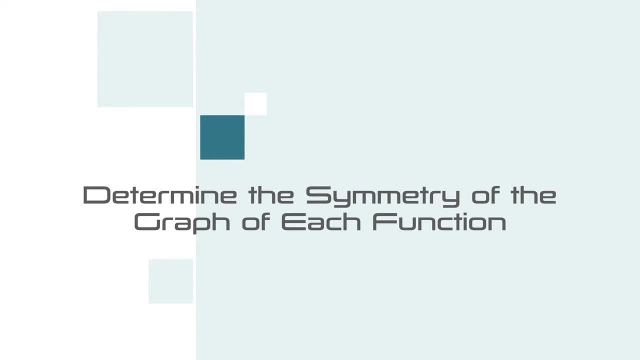 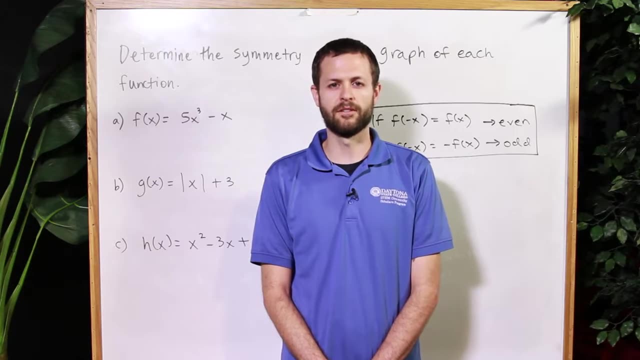 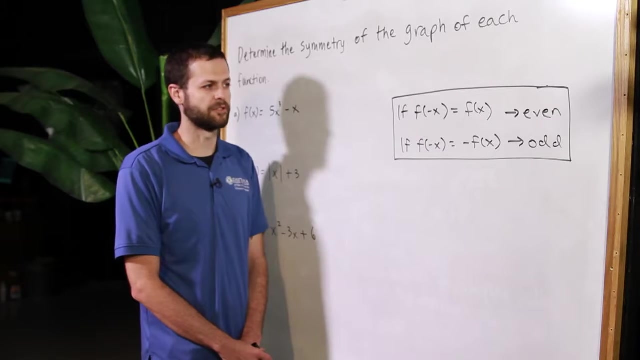 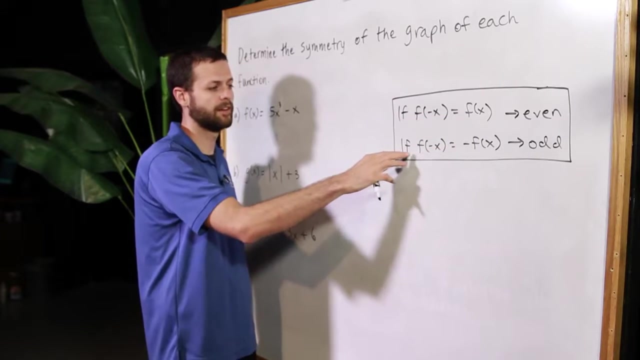 In this problem we want to determine the symmetries of graphs of functions. First of all, what I want to note is the test for symmetries of graphs of functions. Remember that if f of minus x is equal to f of x, that function is even. On the other hand, if f of minus, 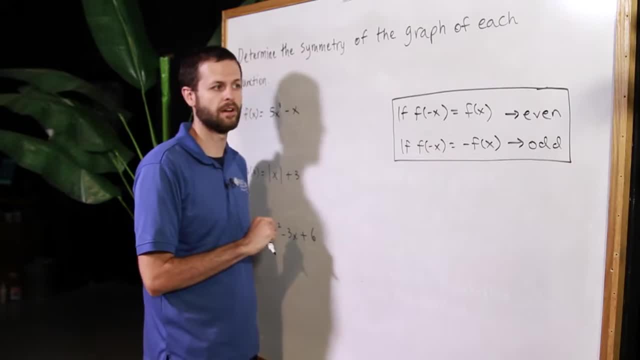 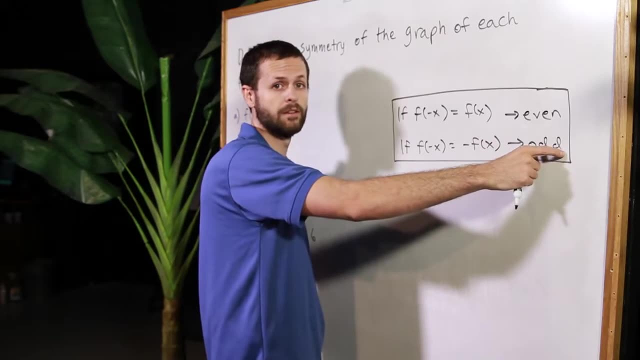 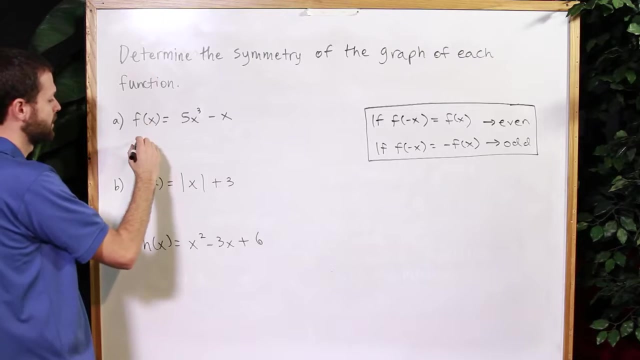 x is equal to minus f of x. that function is odd. Remember that even symmetry means symmetric with respect to the y-axis. Odd symmetry means symmetric with respect to the origin. First of all, what I want to do is, wherever I see an x, I want to put in a minus. 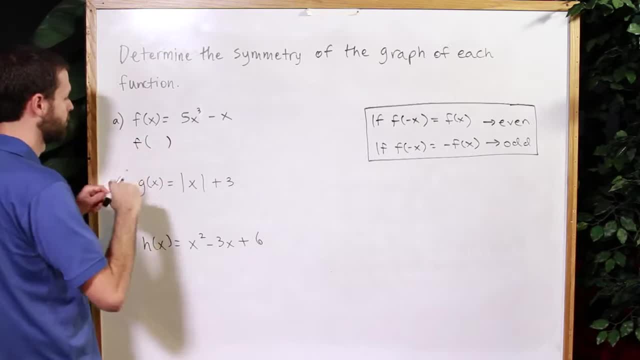 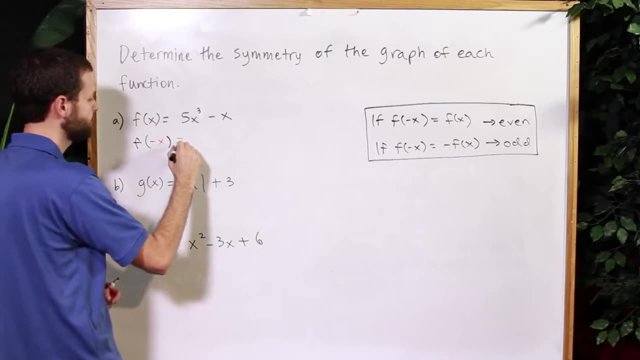 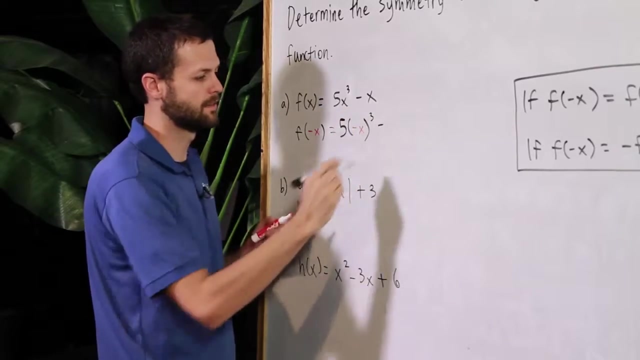 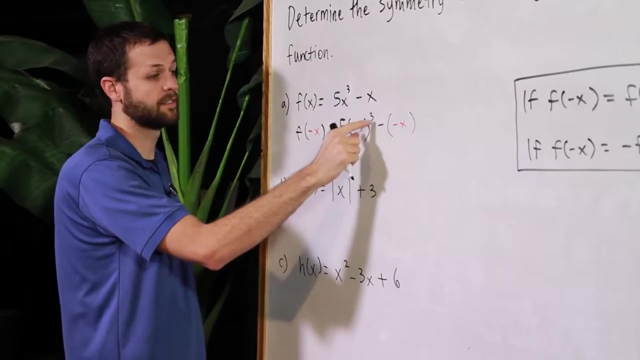 x. This will help me figure out whether my function is even or odd and then be able to determine whether it's symmetric with respect to the y-axis or the origin. This becomes 5 times minus x cubed, minus a negative x. First of all, notice that negative x cubed. 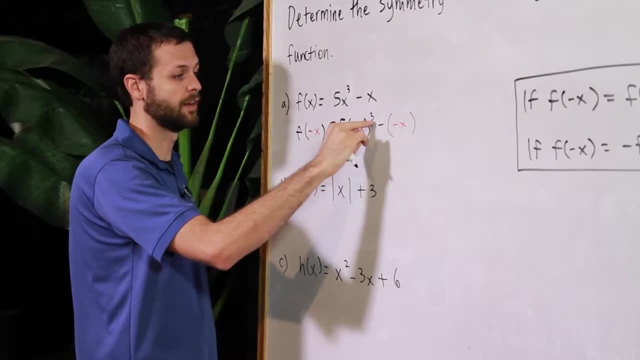 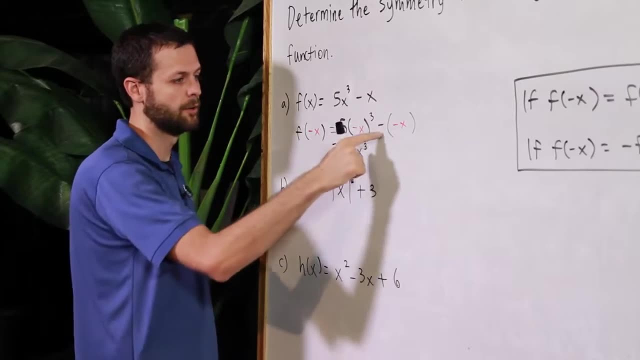 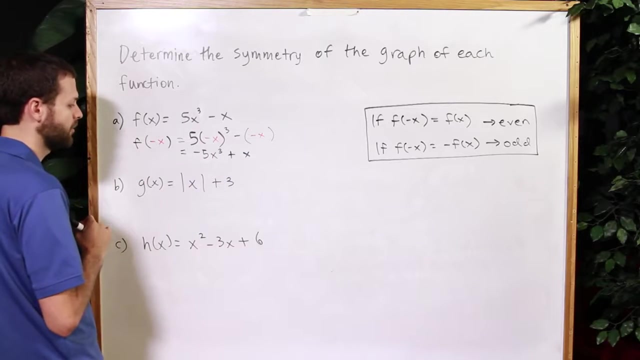 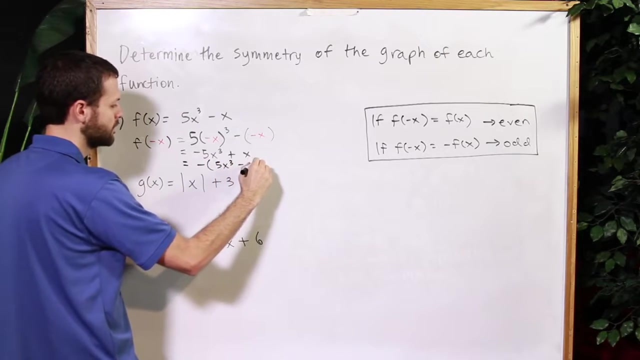 that's just negative x cubed. In other words, a negative to an odd power is still a negative, So I get minus 5 x cubed. upon simplifying Negative times, a negative is a positive, so plus x. What I can then do is factor out a negative, so this gives me minus 5 x cubed, minus x. 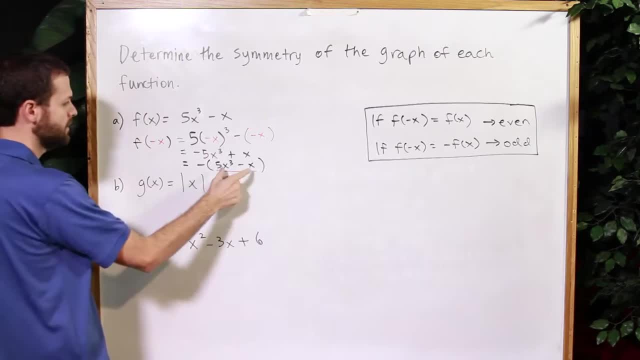 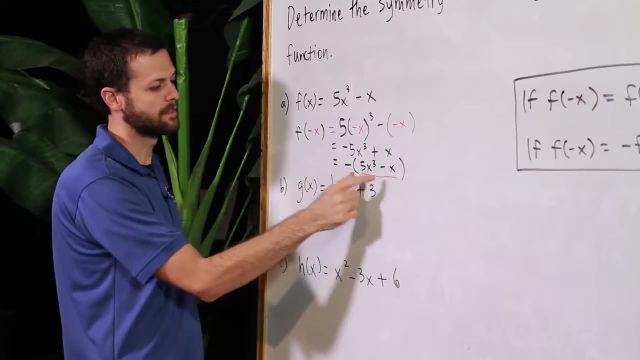 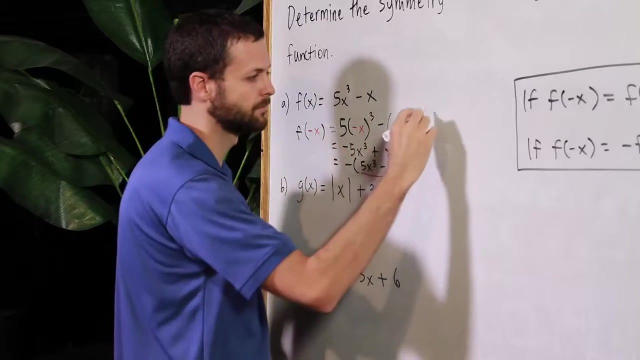 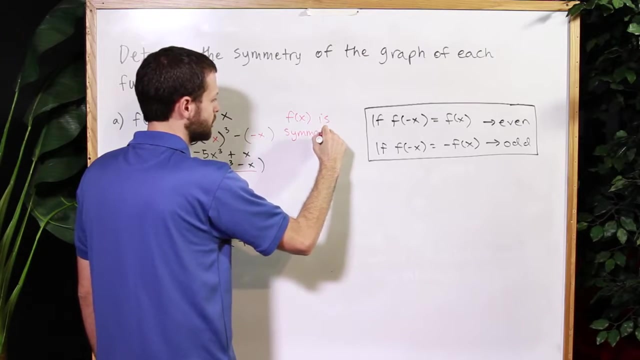 Notice that this part right here. this is the same as my original function. So what I've just proven is that f of minus x is equal to minus f of x. So this function must be odd or symmetric with respect to the origin. I will use the abbreviation WRT to mean with respect to the origin. Let's apply the same. 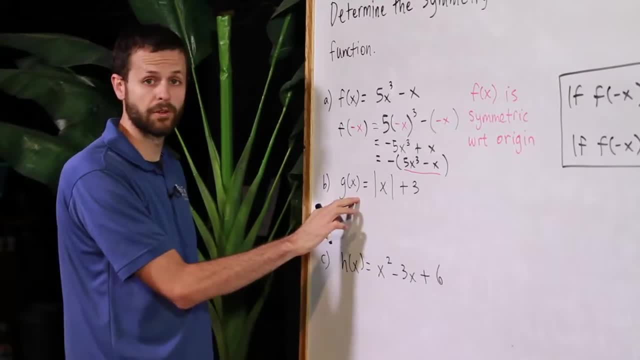 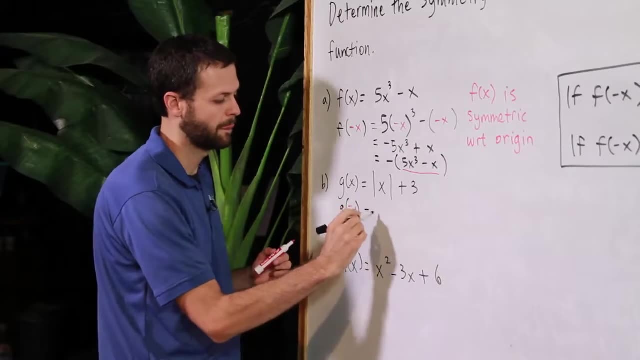 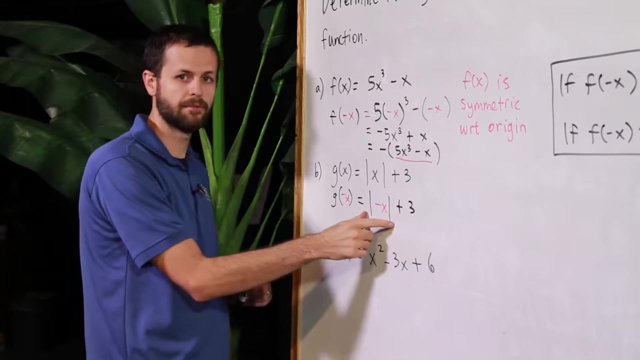 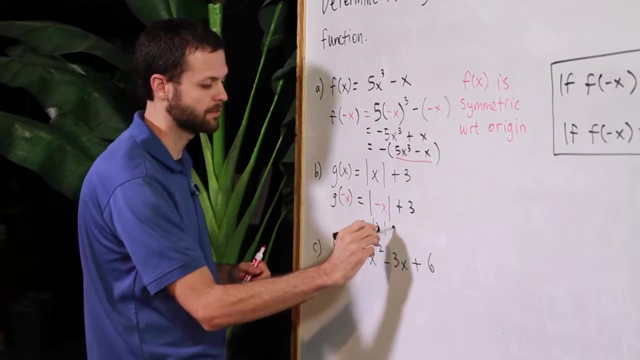 test here for g of x. Again, wherever I see an x, I'm going to put in a minus x. So this Notice that the absolute value of minus x is just the same thing as the absolute value of x. So what I in fact have is the absolute value of x plus 3.. 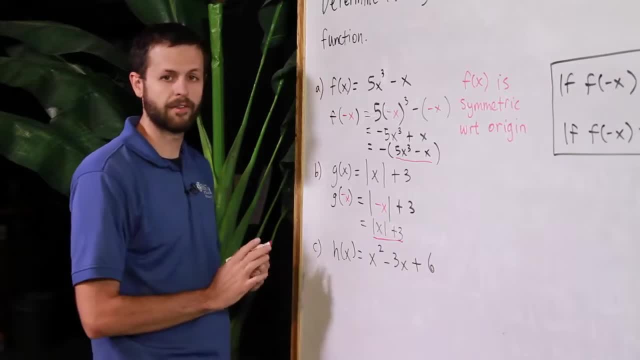 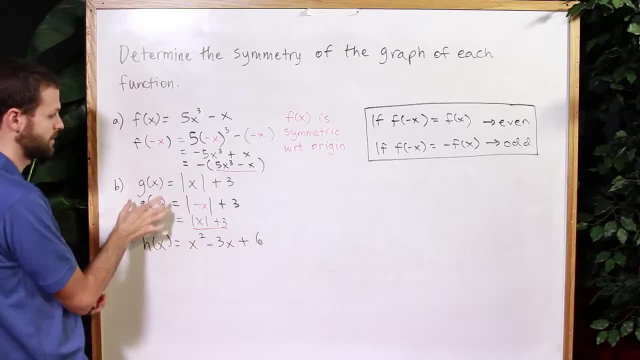 And notice what we have here: Absolute value of x plus 3 again, which is the same thing as the original function g of x. Therefore, since f of minus x- and f in this case is my g- g of minus x is the same thing as g of x. 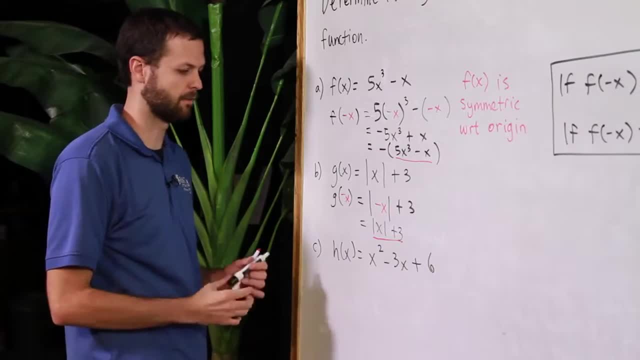 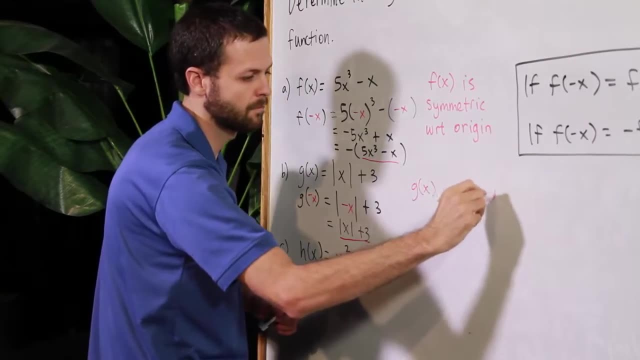 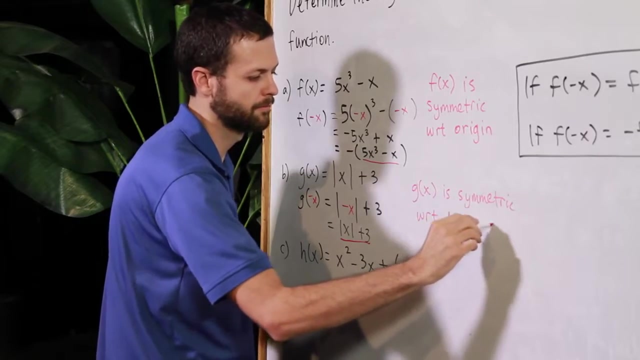 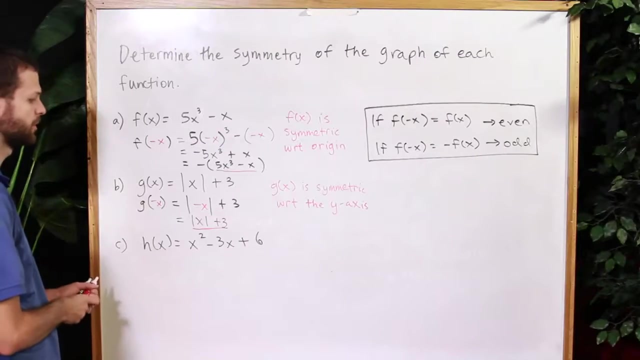 we're dealing with an even function which is symmetric with respect to the y-axis. I'll use the abbreviation wrt to mean with respect to. And finally, we have h of x. Again, what I'm going to do is, wherever I see an x, I'm going to put in a minus x. 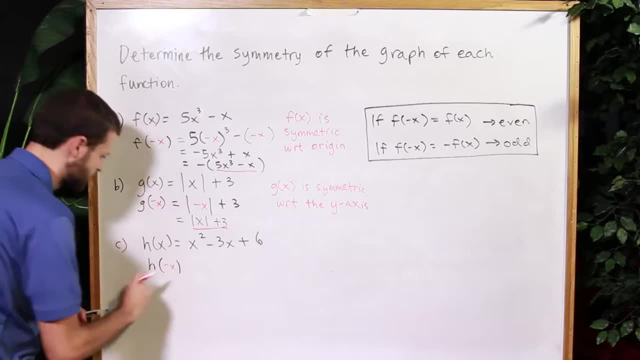 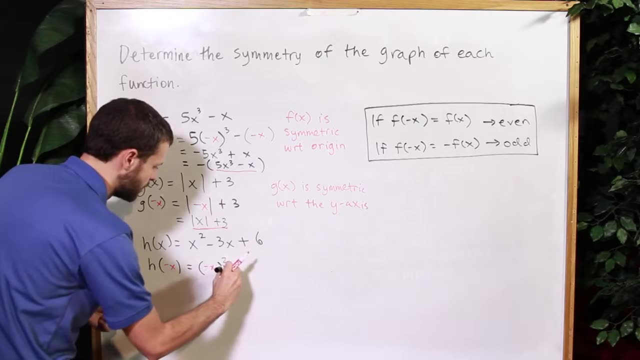 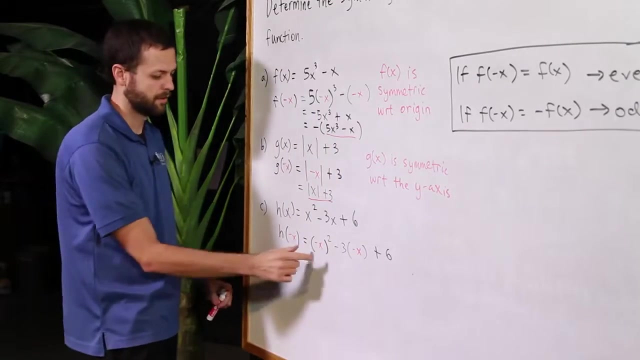 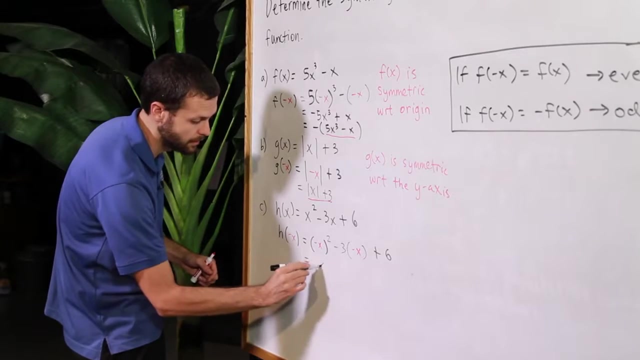 Now I have minus x squared minus 3 times minus x and plus 6.. So let's see what we come up with. Minus x squared- that's the same thing as positive x squared. Negative 3 times a negative x, that's the same thing as plus 3x. 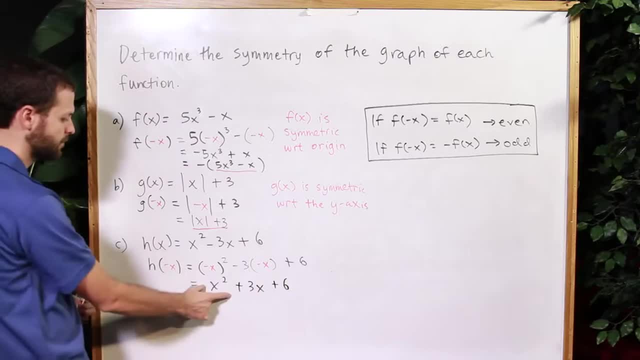 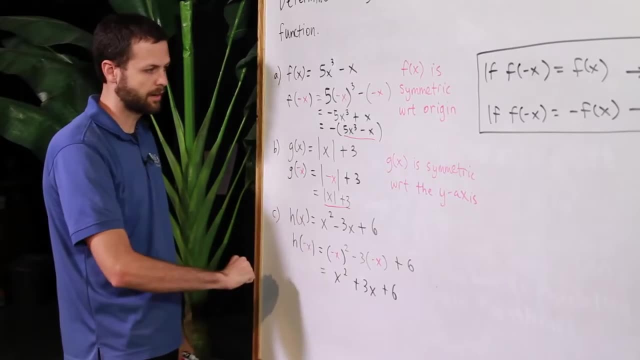 And then I still have this plus 6.. So I have x squared plus 3x plus 6.. Well, notice that that is not the same thing as h of x. And if I were to factor out a negative, like I did here, 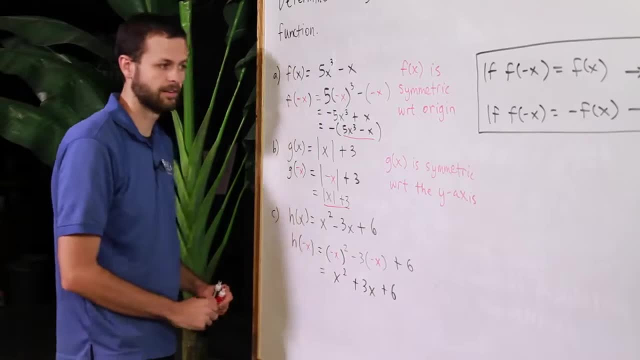 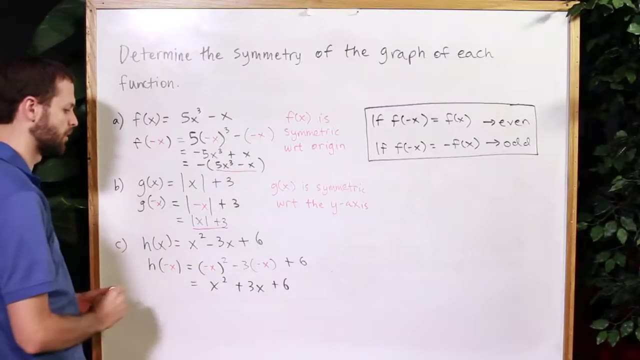 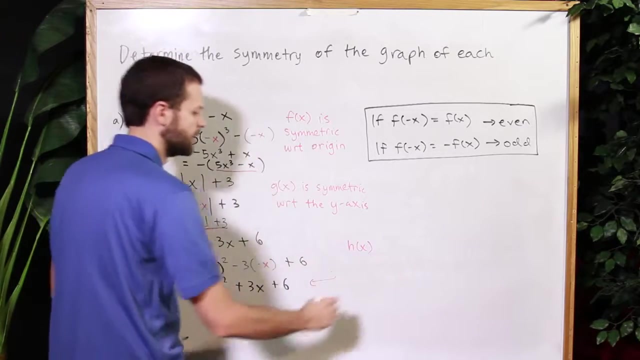 I still wouldn't have h of x on the inside. So in fact this function is neither odd nor even meaning. it has no symmetry about the y-axis or about the origin. So we would say h of x is neither odd nor even. 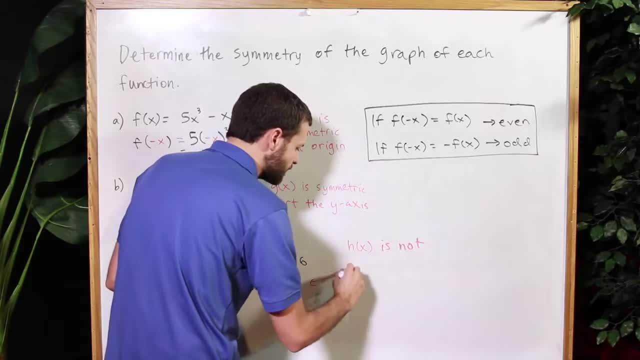 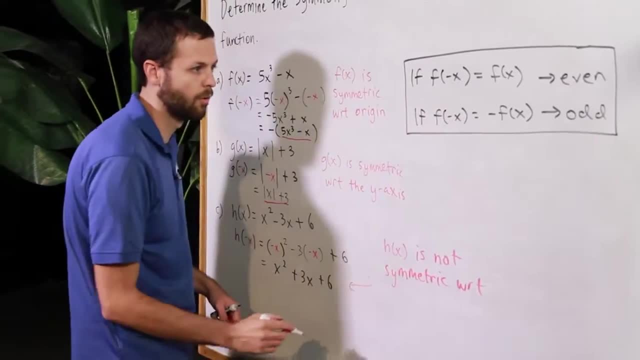 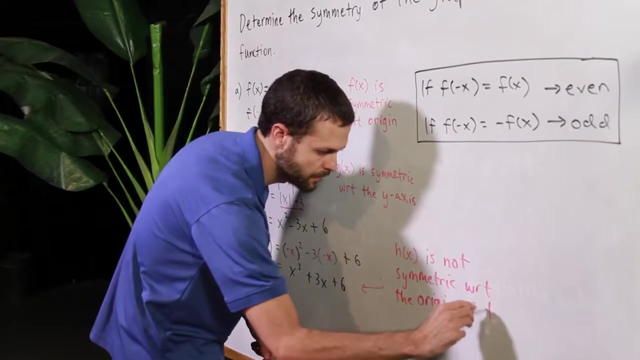 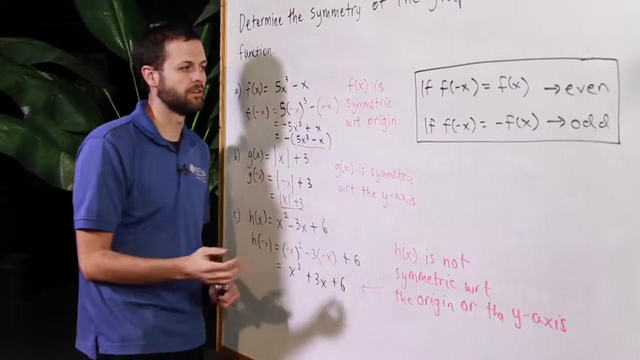 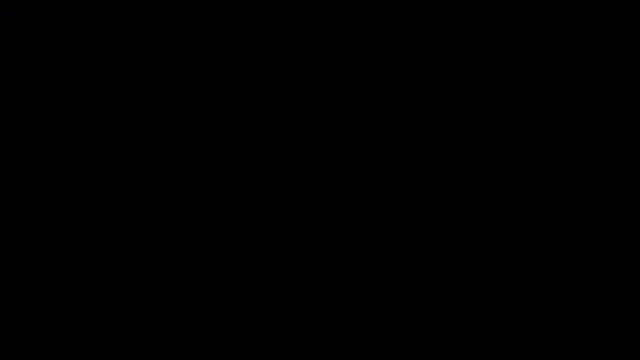 So h of x is not symmetric with respect to the origin or the y-axis. Using these two simple tests again is very important in order to determine the symmetry of a given function and whether that function is odd or even. Thank you,